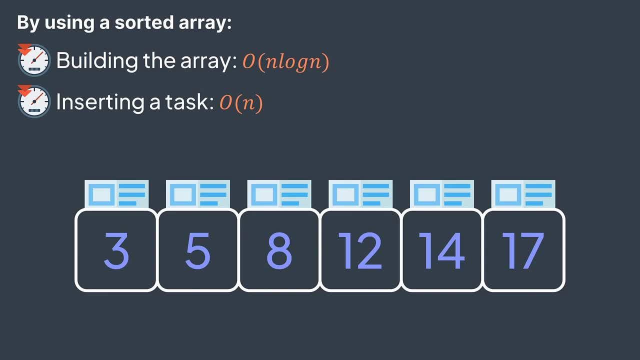 search, you'd still need to maybe shift elements, which causes off and time complexity. What's the solution then? Well, we have this data structure that you will learn about today. that is called the heap. The heap is a tree data structure where each node is smaller. 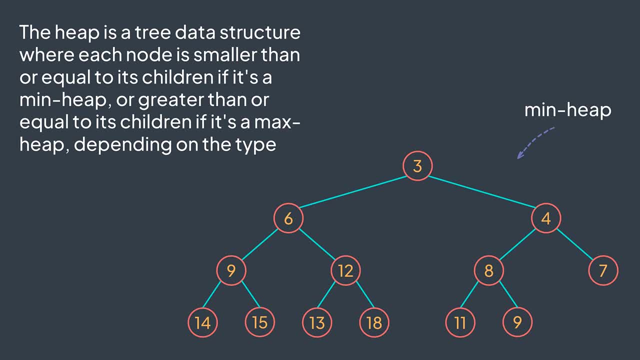 than or equal to his children If it's a min heap, or greater than or equal to his children if it's a max heap, depending on the type. For example, the one on the screen is a min heap And because the root is smaller than or equal to his children in case of min heap. 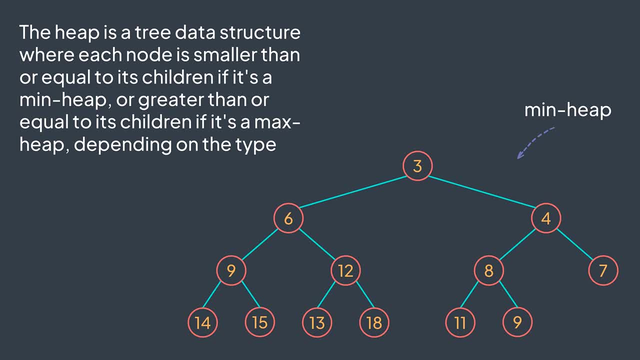 and his children are also smaller than or equal to their children, And so on. then the root is smaller than or equal to all the nodes in the heap Hence the root is always the smallest element. Same logic for max here, but with the word greater. 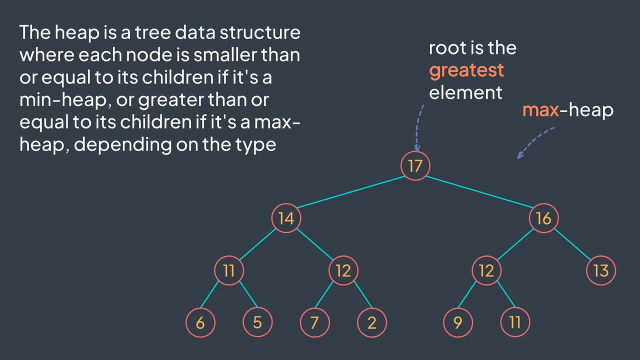 We did use that. getting the smallest or greatest element in a min heap or max a perspective leak costs of one, because we know that is the root, is a great advantage. We have different variants of the heap. we have the binary heap, the Fibonacci heap, the two, three heap and 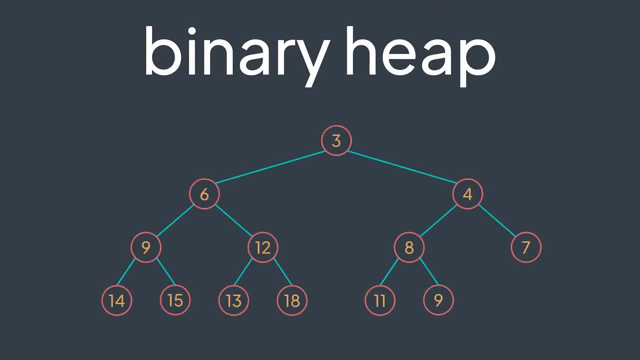 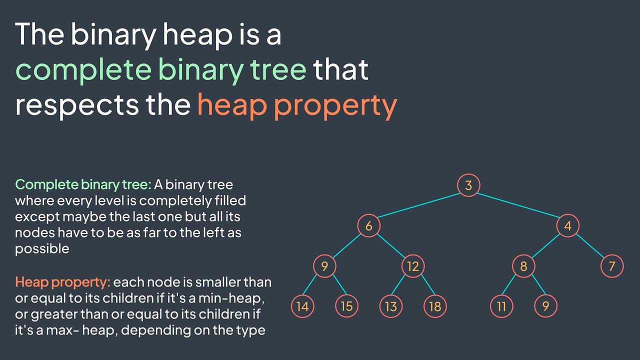 the binary heap. Today we will study the most famous one binary heap. The binary heap is a complete binary tree that respects the heap property. A complete binary tree is basically a binary tree where every level is completely filled, except maybe the last one, but all. 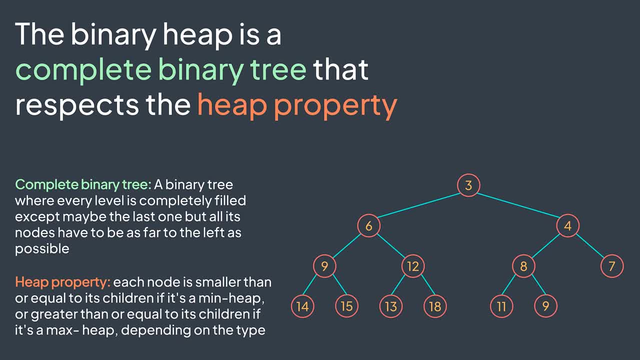 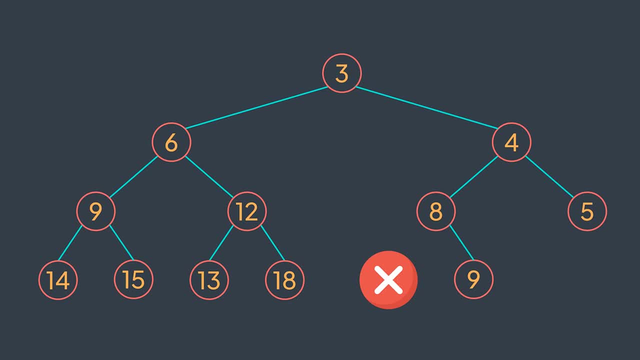 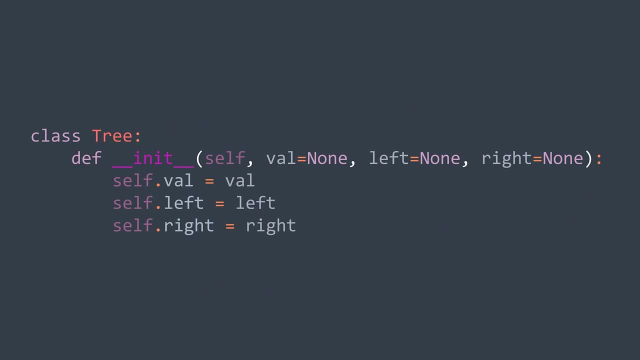 its nodes have to be as far to the left as possible. So we can neither have a null value in a non last level nor null value before node in the last level To store a binary tree we usually have a tree class Or something like that. But when the binary tree is complete, like for the binary heap, 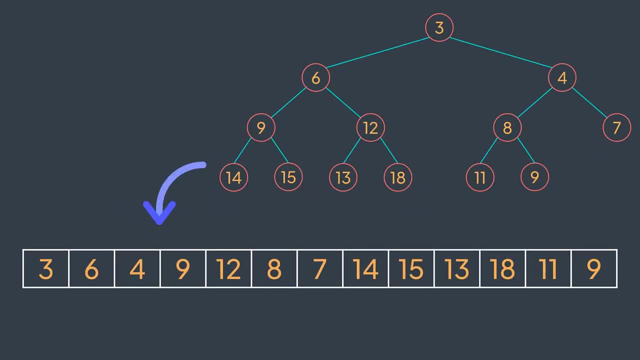 we can just store it in an array, which is more efficient. Why? Because when a binary tree is complete, we have no problem to find the related nodes. when we store it in an array, For any node of the index i, we can find its left child, which is the index two i plus. 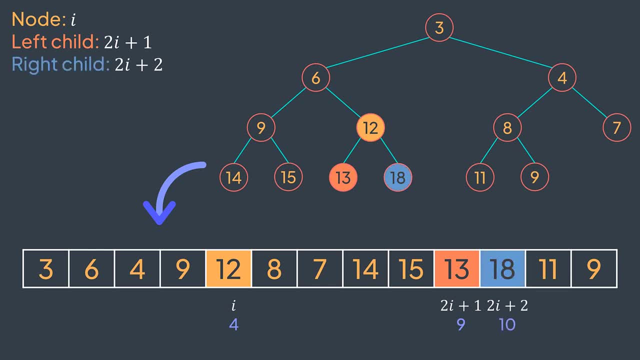 one, its right child, which is the index two i plus two, and its parent, which is the index i minus one divided by two. Therefore, we can easily move between the nodes just by calculating the index, And that's what we'll do when we implement the binary. 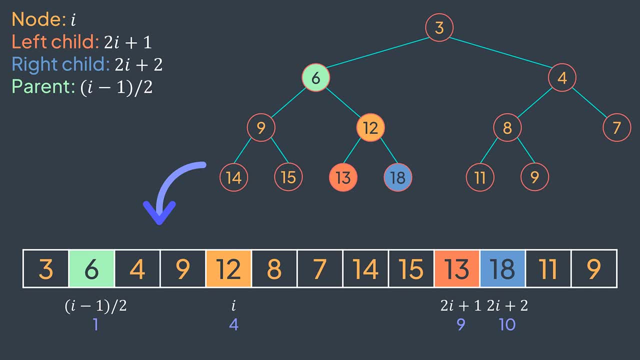 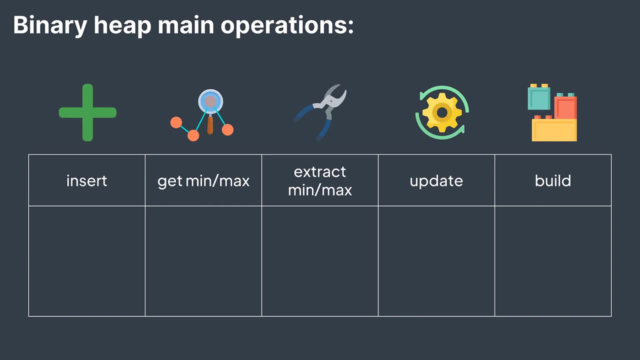 heap. we will store it in an array, but I will still show you the true representation to understand what's happening. We have five main operations that we need in a binary heap: want to be able to insert an element, get the min or max element, extract the min or. 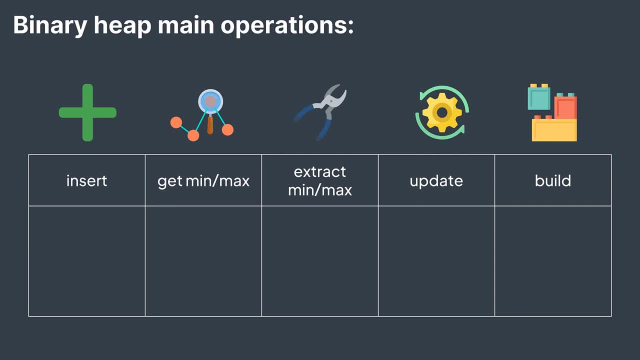 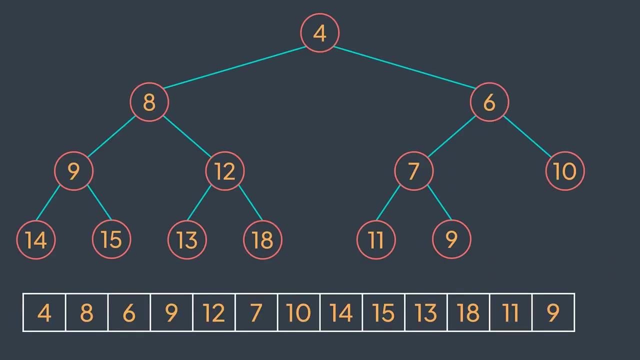 max element, which means getting its value but also removing it from the heap. update the value of a node and build a heap. You need to know that we cannot add, update or remove a node from a heap randomly. we need to respect the heap property. For example, if we have this min heap and we insert five, 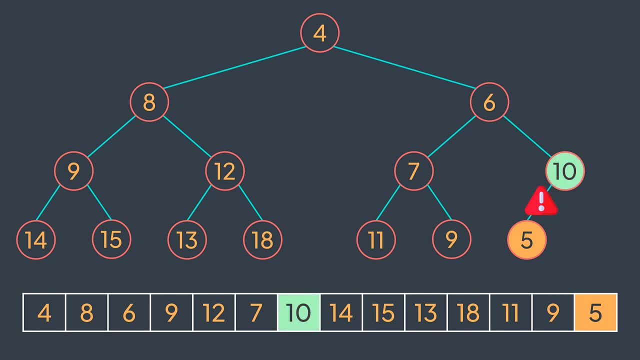 without doing anything else, we would break the heap property. 10 is not smaller than or equal to his children anymore. To respect the heap property we need to apply an operation called sift. We have two sift operations. we have sift up and sift down. When the node 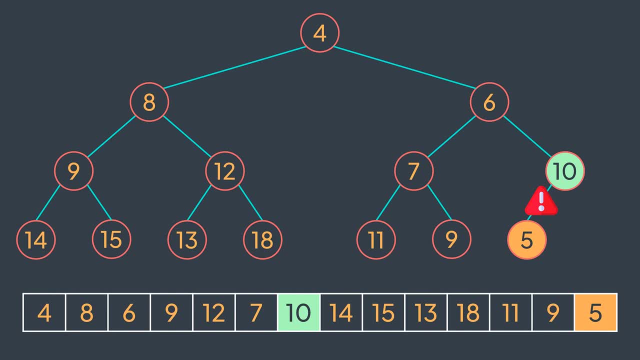 that we want to reposition is at the bottom, we'll apply sift up, And when it's at the top, we'll apply sift down. And sift up will keep swapping the node with its parent while smaller, For example, with the five here it's more than its parents always wrap, It's. 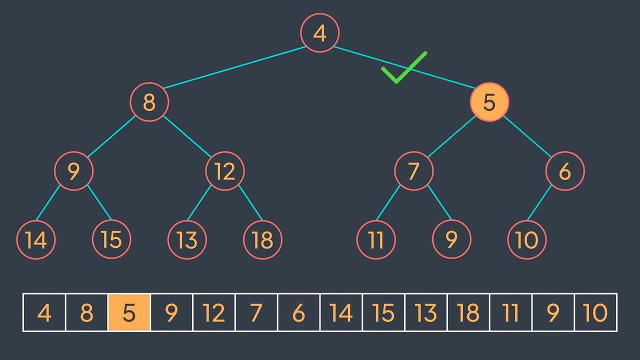 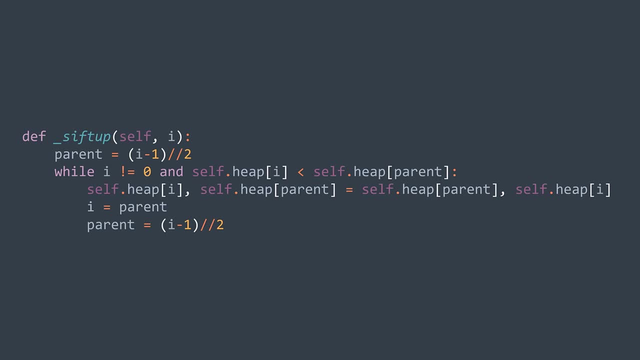 still smaller than its parents always wrap. It's not small anymore, So we stop. the heap property is respected again In code. who want to sift out the element at index i? so we calculate the index of its parent as shown earlier. then why it didn't become the root. 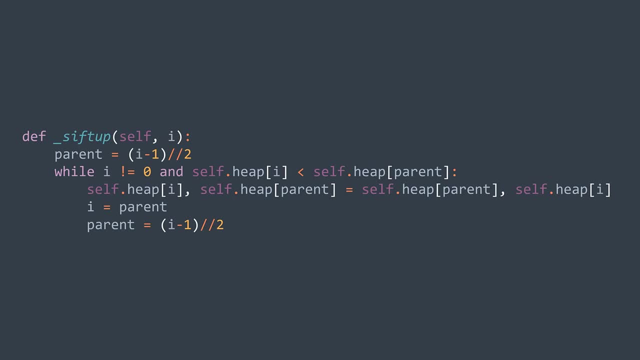 or it's more than its parent. 12 note: I was its parent and I becomes parent index because it took its place in the heap. We also recalculate the parent index for the next iteration. That's it For sit down. we keep swapping the node while it has a smaller child, If both are smaller. 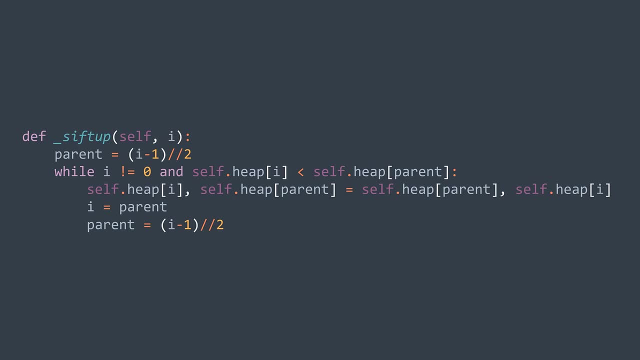 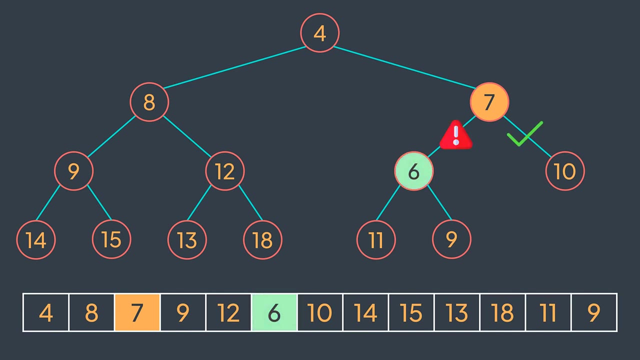 we swap with the smallest one. For example, if we want to save down seven in this heap, it's right child is smaller, So we swap Now. it's left child is smaller, So we swap Now. both are not smaller. So we stopped. he properties respected again In code. we want to sift down. 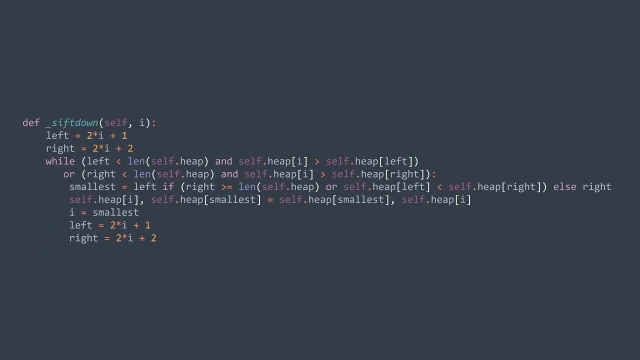 the element that index. I start by calculating indexes of left and right children, as shown earlier. Then, while the node is greater than one of them, who start by determining the smallest one? the smallest one is the left child if the right one doesn't exist, or the left one is smaller. 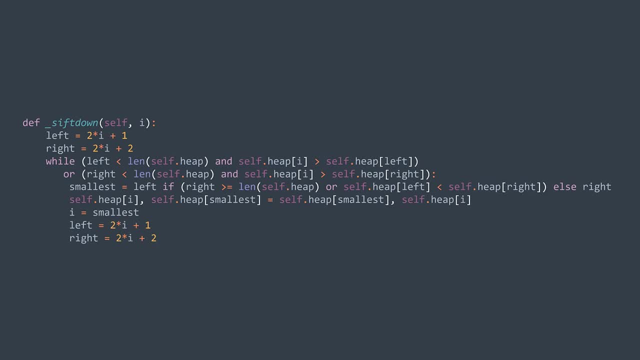 than it Else. the smallest one is the right child. Now that we found the smallest, who swap between it and the node, I will update the index- I because it took the place of the smallest- and recalculate the indexes of left and right for the next iteration. That's it, And in both of these operations, at each. 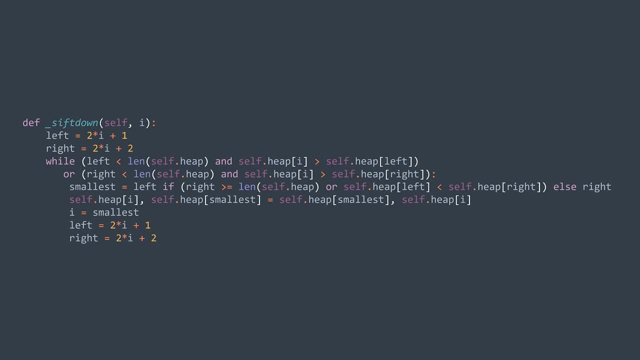 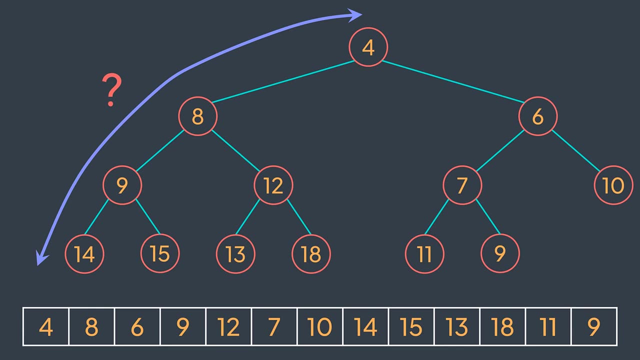 iteration, the node moves by one level in the heap, So the number of iterations depends on the height of the heap, And because the binary heap is a complete tree and a complete tree is always balanced, Then the height is an off log n, where n is the number of elements in the heap. 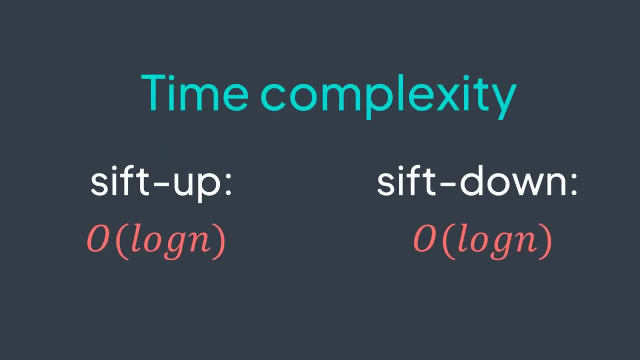 So the time complexity of sift up and sit down is off. log n: Okay, we know how to sift up and sit down, But why do we need these operations? We need them to insert, update and delete elements, as we will see now. 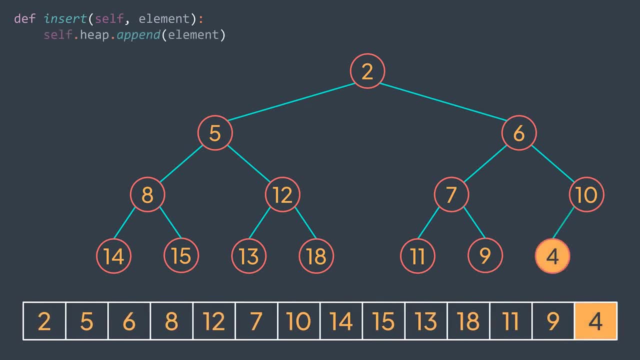 To insert an element in a heap, we just need to insert the value at the end of the array. But it may break the heap property, So we apply sift upon it to take it to the right place. Sift up, because it starts at the bottom of the heap. 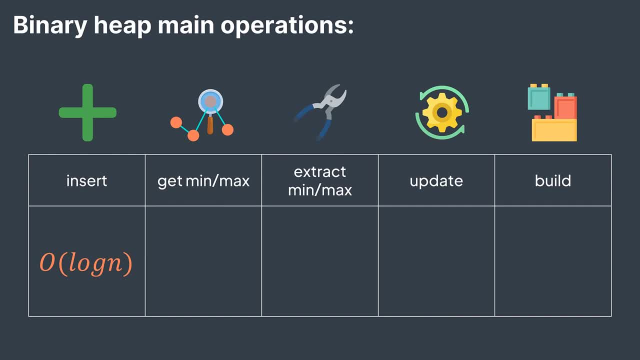 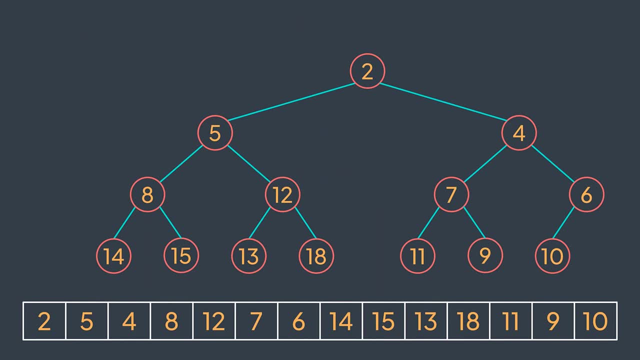 And this operation has an off log n time complexity because we're calling sift up. The second operation is get min And we know that in a min heap the smallest element is always at the root, which is the element that index zero in the array. So we just return heap of zero. 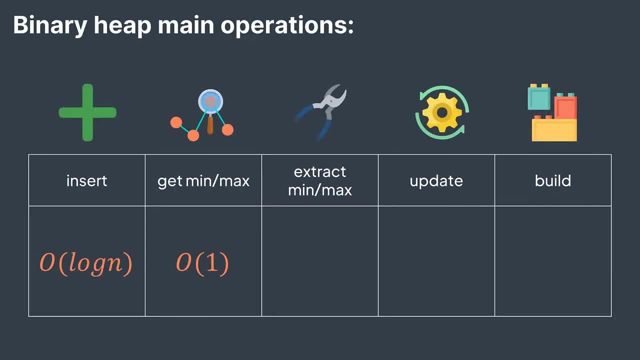 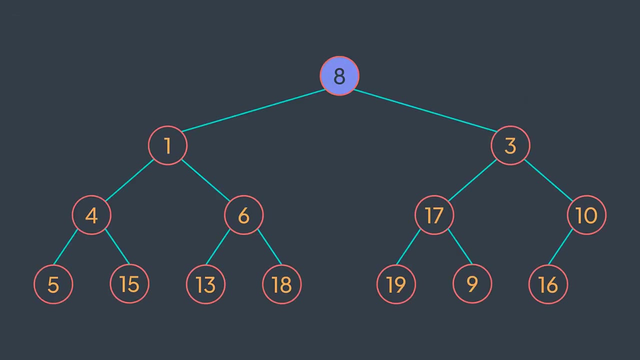 if it exists. Obviously we get an old one time complexity for this operation because we already know the index. Next operation is extract min. Here we want to get the minimum value, but also to remove it from the heap, First of all in the tree. we can't just delete the root darkly, because his children 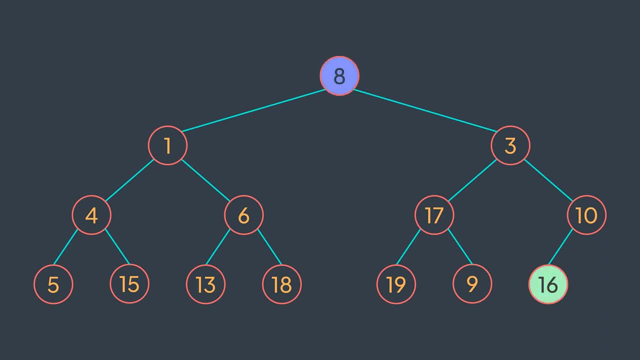 would have no parent. What we do is that we first swap it to the leaf node and we delete the No, that was the root previously. it gets safely deleted because it's a leaf, it has no children. And in heap we do the same thing to delete the root, which is the smallest element we first swap. 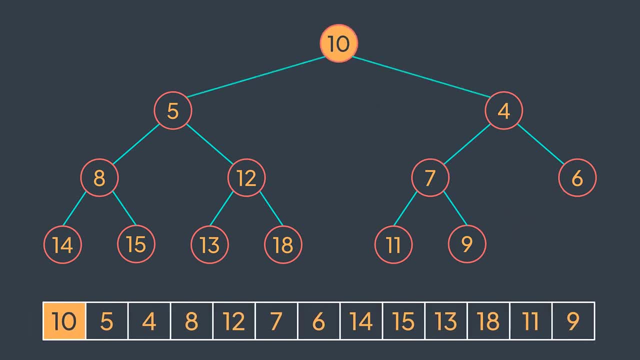 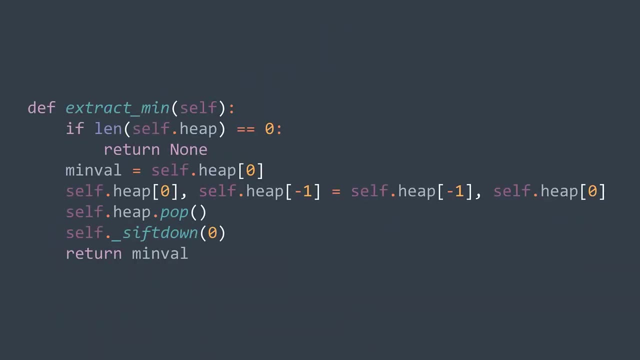 it with a leaf. we swap it with the last element in the array and we pop to remove the node. But this operation may break the heap property. So we apply save down on the new route to take it to the right place. save down because the route is other top In code. we first check that the 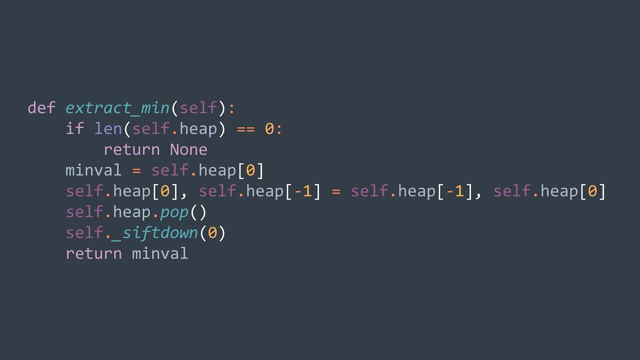 heap is not empty, then we save the value of the smallest element because we will need to return it later. Now we swap the route with the last element and we pop to remove the node. We also save down the new route- it's at index zero- and return the main value. The time complexity is also a flow and 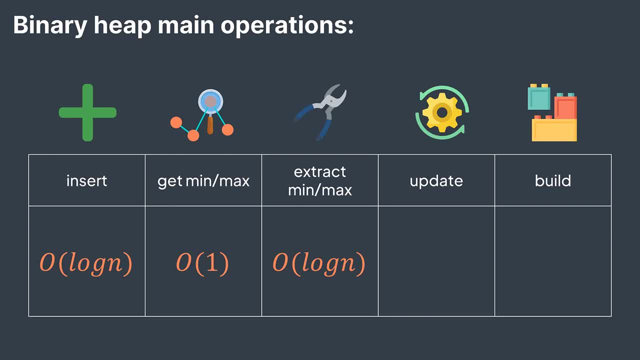 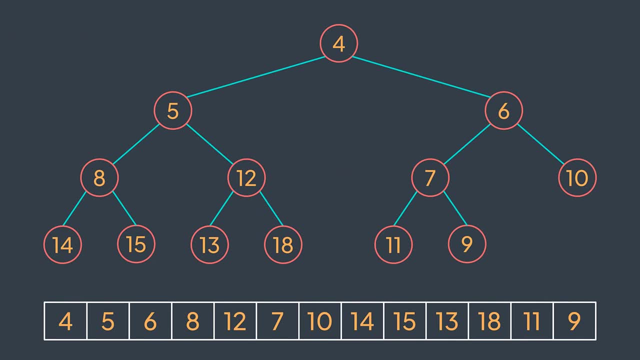 because we're calling sift down Next operation updating the value of a node. we actually have a structure that respects the heap property, But if we update the value it may break the heap property. So we have to sift To know if we should sift up or sift down the updated node. we compare 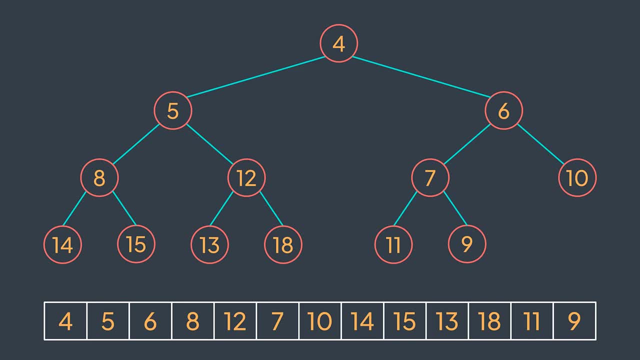 the old and the new value. If the new value is smaller, we have to sift up or down the updated node. We compare the old and the new value. If the new value is greater than the node may need to go up. So we sift up Else if it's greater than the node may. 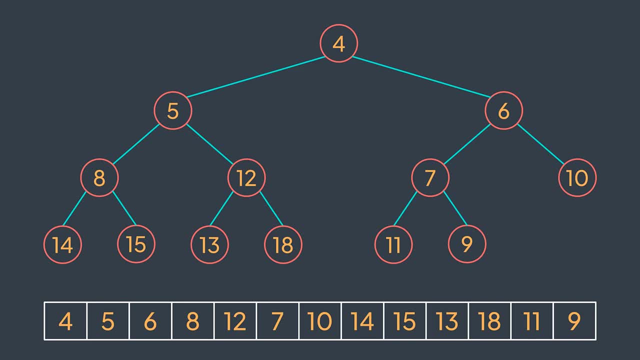 need to go down, So we sit down. Let me show you two examples. Let's update seven with two. The new value is smaller, So we sift up to a smaller than its parent. six, So we swap. It's still smaller than its parent, So we swap. Now we stop because it became the root. 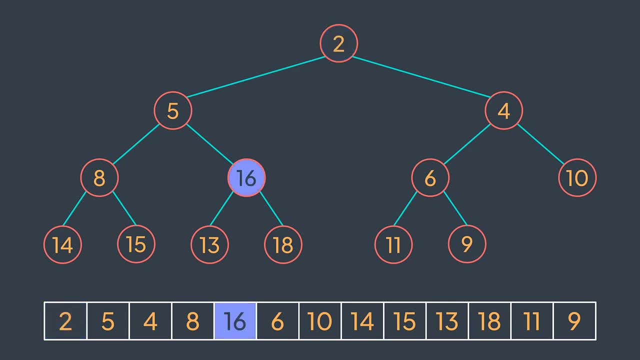 Second example: let's replace 12 by 16.. The new value is greater, so we sift down. 16 is greater than its left child, So we swap. It has no children anymore, So we stop the heap properties respected again In code. it depends on if we have the index of. 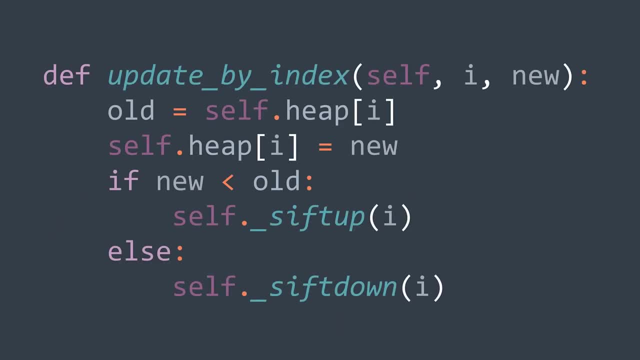 the element that we want to update or not. If we do, we do save the old value to compare later. we update heap of i by assigning the new value. then we compare. If new is smaller than old, we sift up, else we sift down. This operation costs of log n because of sifting. 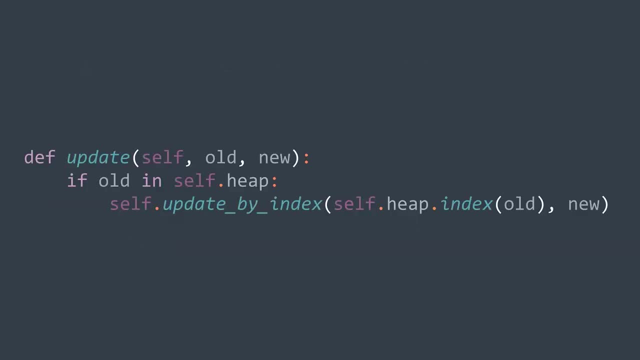 But if we don't have the index, we first need to find the index of the element that we want to update. So if it exists in the heap we search for its index. then we call the update by index function. we made now This operation costs of n, because we first need to search for the element. 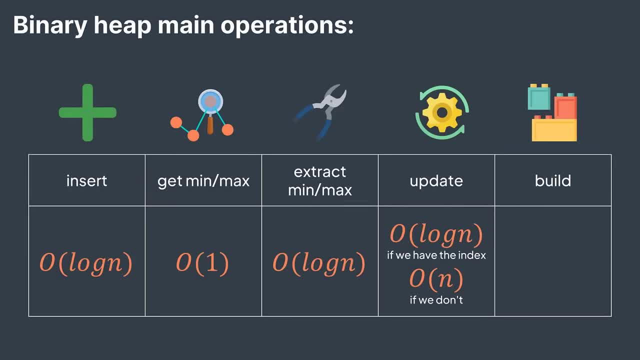 So obtaining an element costs of log n, if we have the index, and of n, if we don't. And last operation, building the heap, also called heapify. The optimized way to do so is to traverse indexes of the array that we want to heapify. 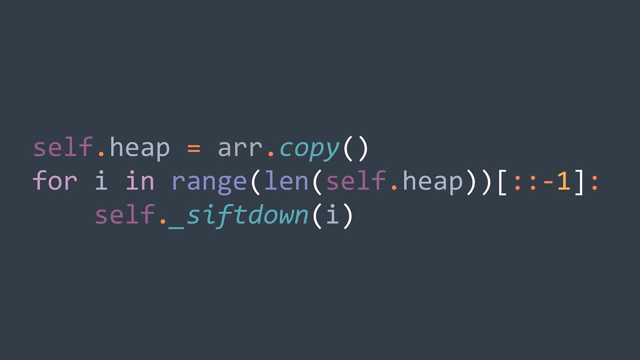 backwards and sift down each element. It's optimized because the cost of sifting down depends on the number of levels between the node and the bottom of the heap, And because we have more nodes that are closer to the bottom, then it's better to use sift down. 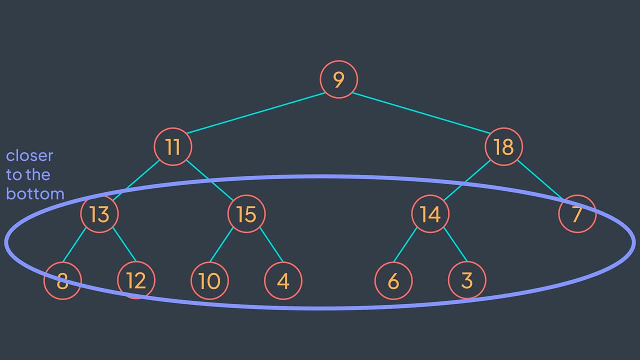 rather than sift up. sift up would need more operations to process the bottom nodes, because they are far from top And who traverse backwards. to start from the bottom of the heap. to avoid sifting down a node and having to do it again later, Let me show you an example. we have this: 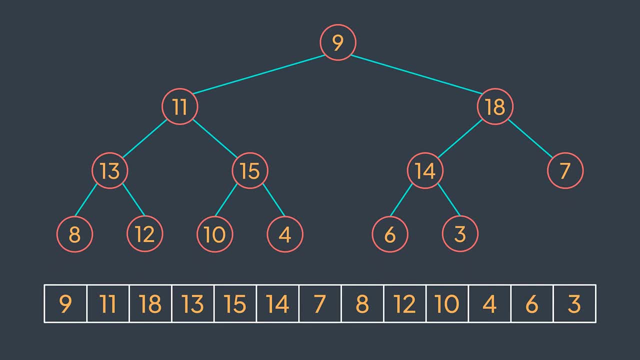 array that represents this binary tree and we want to heapify it. start from the end of the array. The nodes of the last level have no children, so nothing will happen. Then seven: it has no child, nothing happens. Then 14: both his children are smaller. 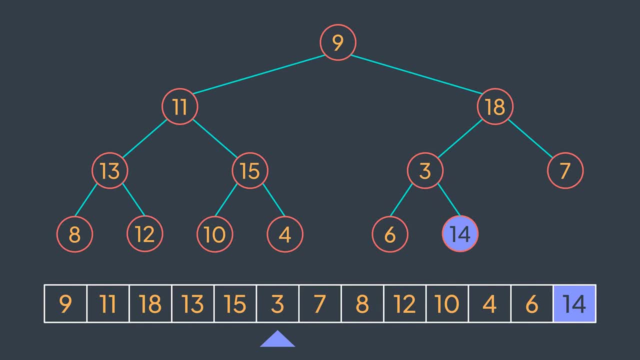 we swap it with the smallest one. Next node 15: same thing. we swap it with the smallest child And it has no children anymore. Next node: same thing. we swap with the smallest one. Next node 18: three and seven are both smaller. who swap with the smallest one? 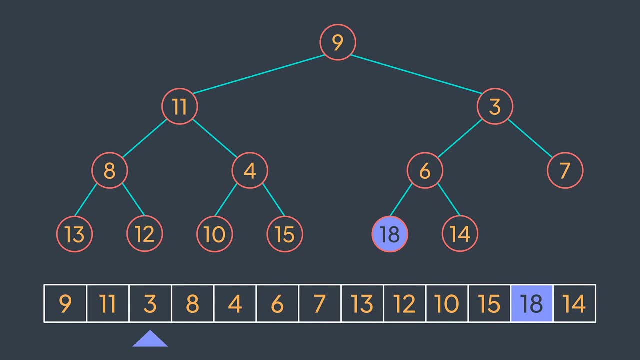 18. still has smaller children who swap with the smallest one. Next node: 11.. It has smaller children who swap with the smallest one. It still has a smaller child who swap. last node: it has smaller children who swap with the smallest one. three: It still has. 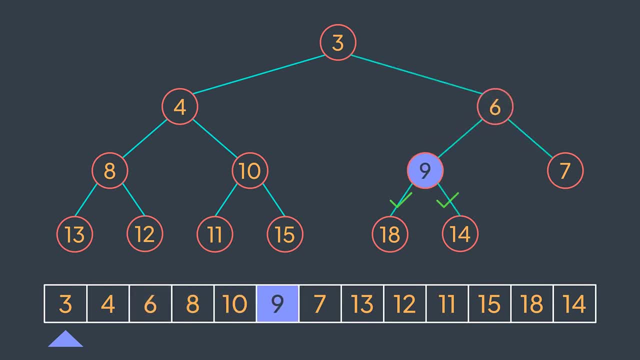 smaller children who swap. Now both his children are greater. we stop swapping And we finished heapy fine. the structure now respects the heap property. What about the time complexity? you need to know that when a tree is complete, the last level has. 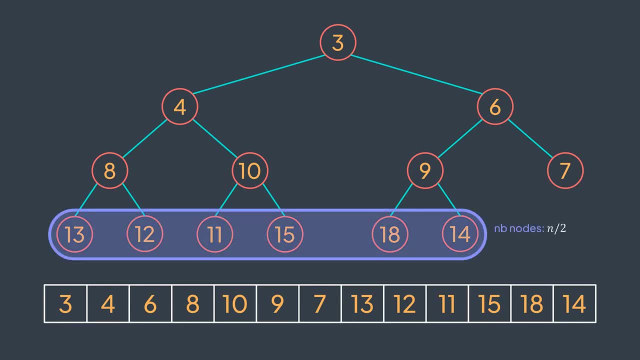 at most around n by two nodes, where n is the total number of nodes. The level above has around n by four than n by eight, and so on until the first level that contains one node, the root, And in sift down, the maximum number of iterations is the number of levels between the level of the actual 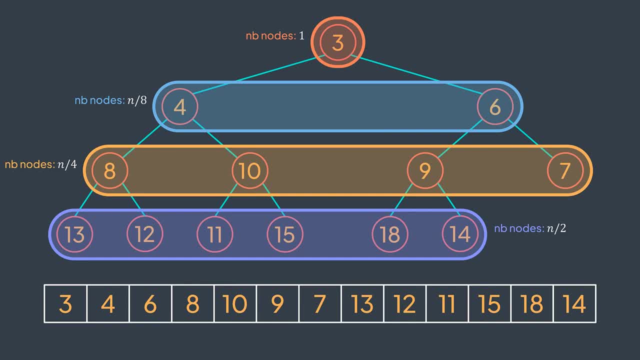 node and the last level. So nodes of the last level are already in the last level. they can't go down. let's say that their cost is zero because we do zero iterations. nodes of the level above do at most one iteration because they are one level far from the last one. let's say that their cost. 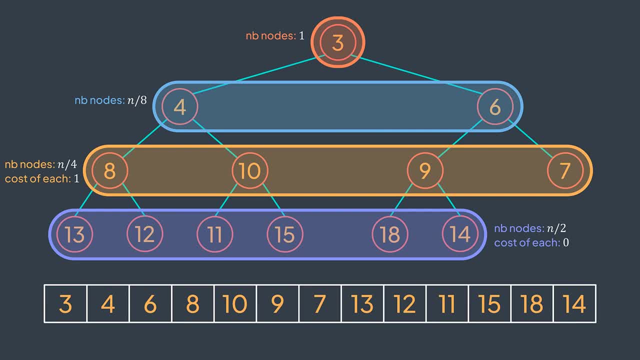 is one, Then the level above is two levels far from the last one. let's say that the cost is two and so on until the root that may require log To have n minus one iterations to sift down And the total cost of heapifying is the sum of each. 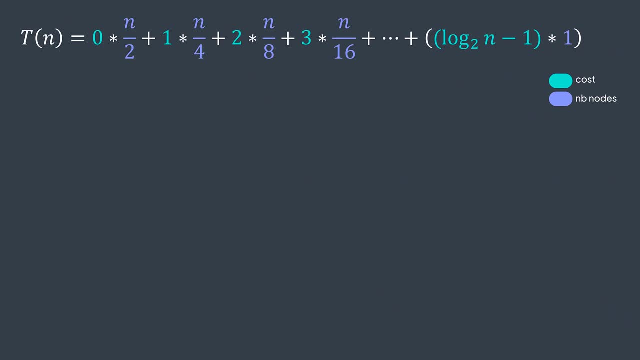 node multiplied by its cost. to sift down, we have n by two nodes that cost zero, and by four nodes that cost one, and by eight nodes that cost two, and so on until one node that costs log two of n minus one. This sum represents the sum of k times n divided by two power k plus one, where k goes from zero. 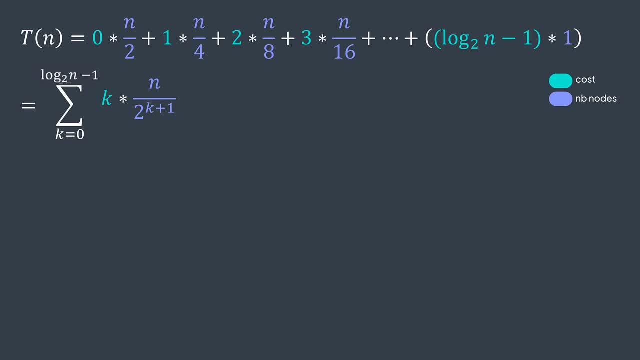 to log two of n minus one. We take n divided by four out of the sums. Now we have n by four multiplied by the sum of k times one divided by two. power k minus one takes some seconds to grasp this. The terms of the series are all positive, So this series is: 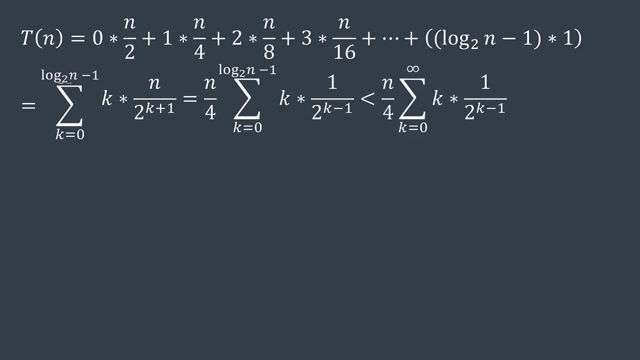 smaller than this one, where k continues to infinity. And it's fun to work with this one because we're searching for an upper bound One divided by two. power k minus one is one. power k minus one divided by two. power k minus one, which we can replace by one divided by two. 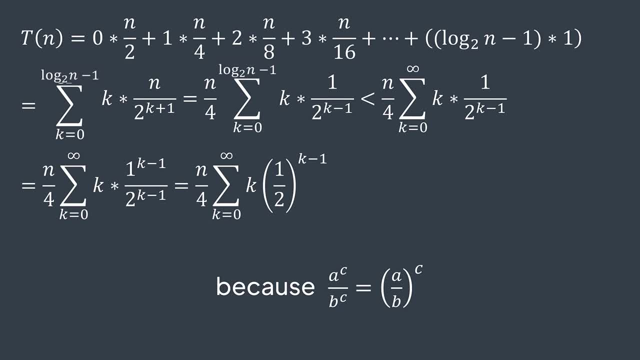 Power k minus one. Now let's replace one divided by two by x, and we notice that k times x power k minus one is a derivative of x power k. we replace, And this series, the sum of x power k, where k goes from zero to infinity, is a known series. its value is equal to one divided by one minus x. 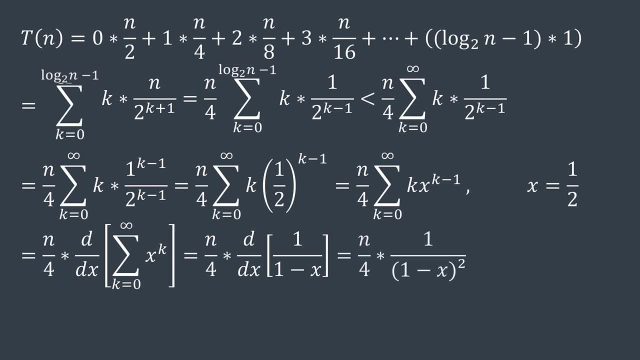 Now we derive one divided by one minus x. we got one divided by one minus x squared. Remember that one divided by one minus x is one divided by two. We replace: one minus one half is one half, and one half squared is one divided by four. Now we have n divided by four times one divided by one divided. 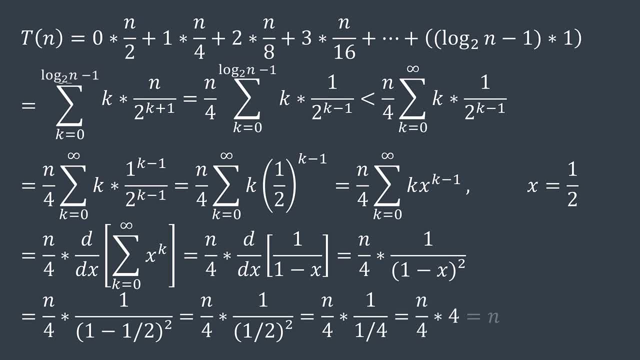 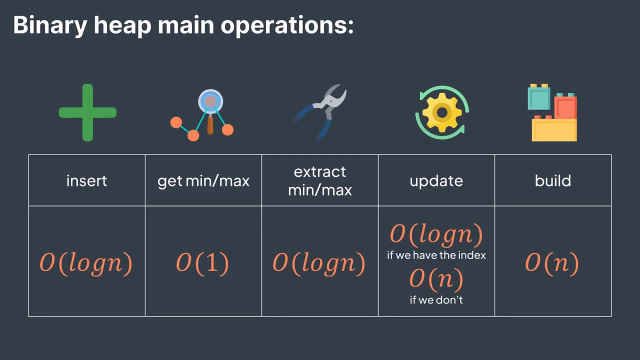 by four, which is equal to n. divided by four times four, which is equal to n, we found out that the cost of heapifying with sift down is n. we get a time complexity of O of n better than O of n log. 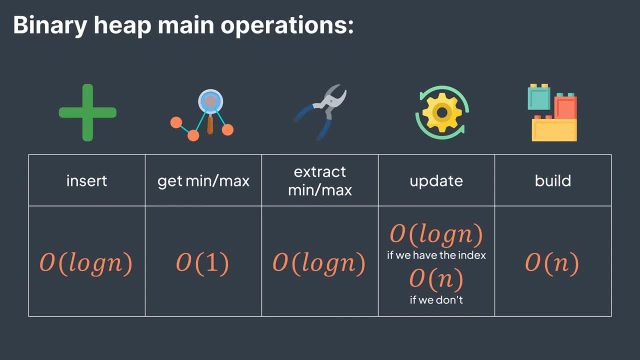 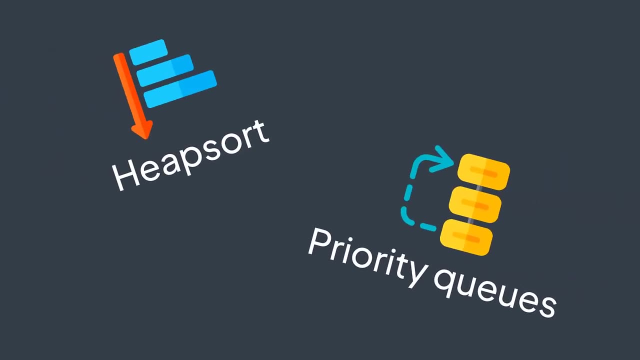 n that we would get if we use sift up. Sift up. Okay, now we know what is a binary heap, its main operations, their time complexity, but where would we use it? To answer this question, let's see two applications of binary heaps: heap sort and 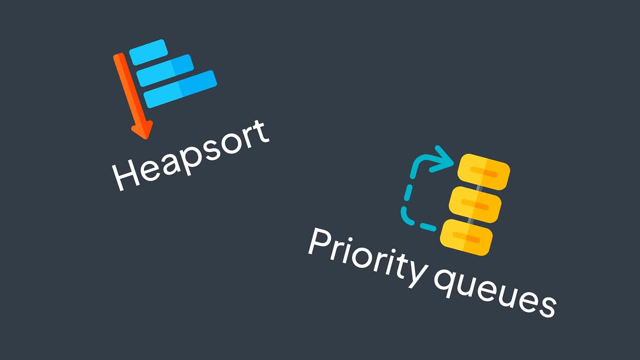 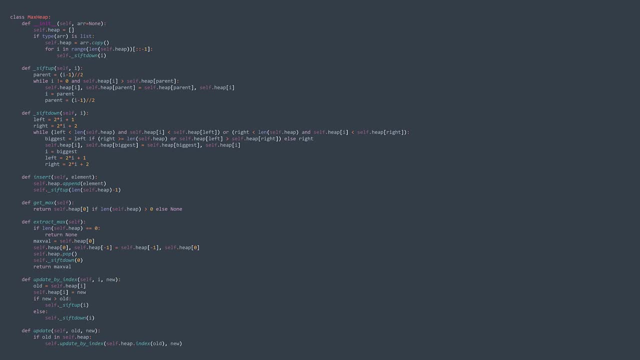 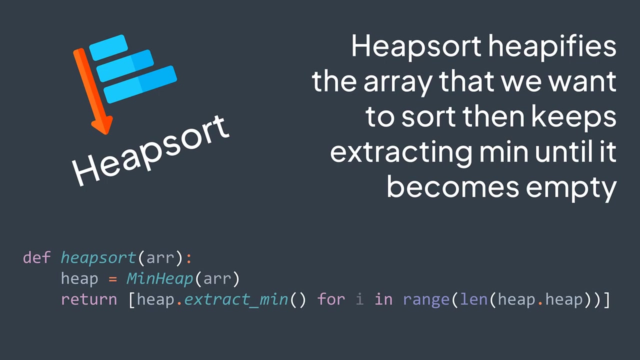 priority queues. But before know that here we implemented the min heap, but implementing a max heap uses the exact same logic. we just reverse the operators and chance on names you'll find the code below. Let's start with heap sort. heap sort is a sorting algorithm that uses a heap data. 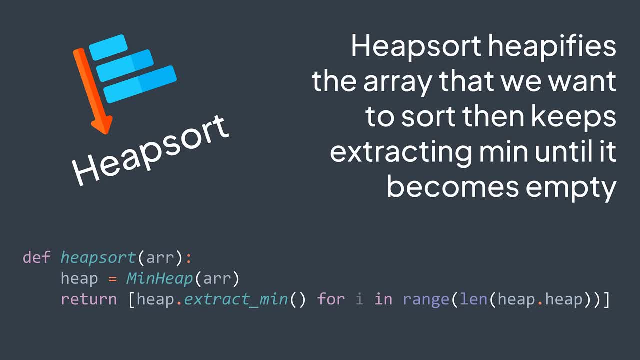 structure It, he finds the array that we want to sort. then it keeps extracting man until the heap becomes empty. That's it. It's like selection sort, where we keep searching for the minimum in the unsorted part. but searching for the minimum in selection sort costs O of n, and we do it n times during. 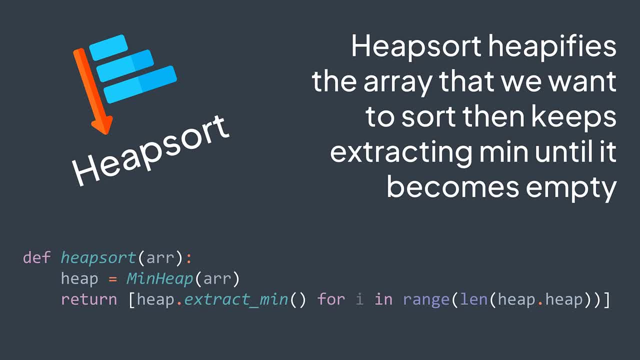 the process. This is why you get an O of n. squared time complexity for selection sort, which is not the case for heaps. So remember that extracting men from a heap cost O of log n only, not O of n. This is why we'll get an O of n and log n. This is why we'll get an O of an log n. 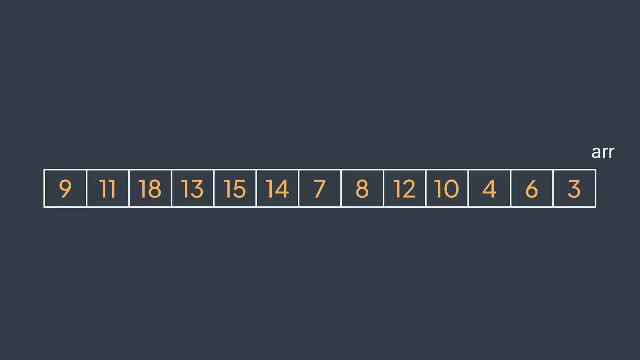 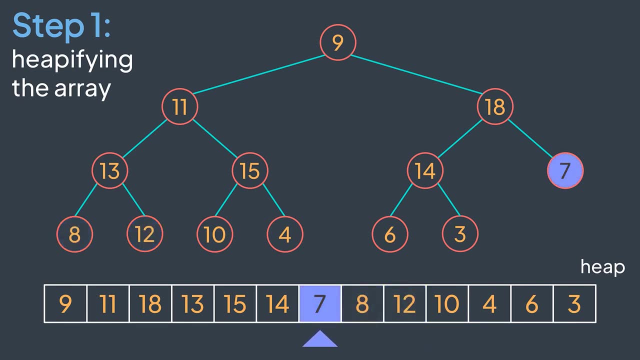 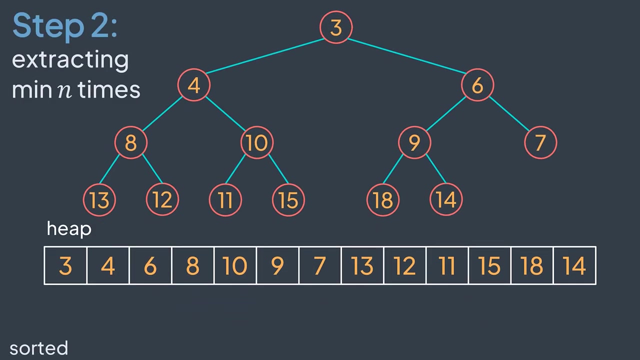 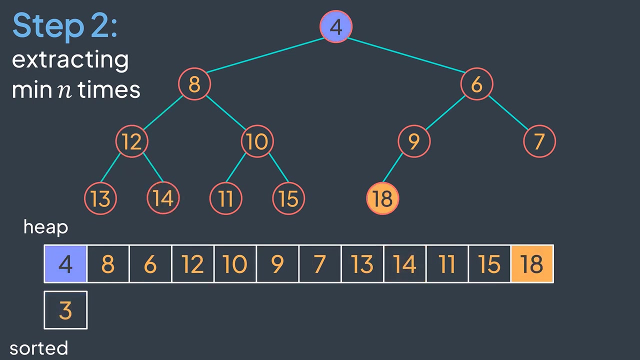 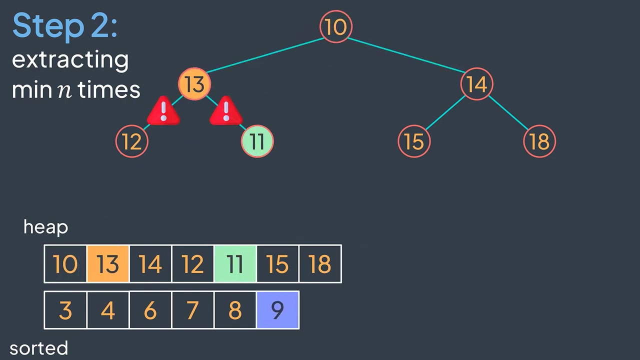 only not of n. This is why we'll get an O of n log n by A. So we'll get a minute of time. complexity, time complexity. Here is an example and what happens when applying hip sword. Here is an example and what happens when applying hip sword. 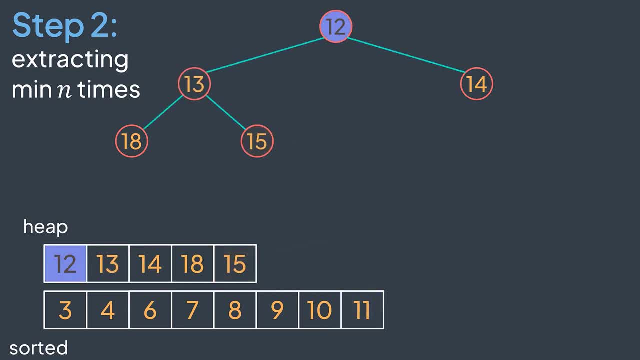 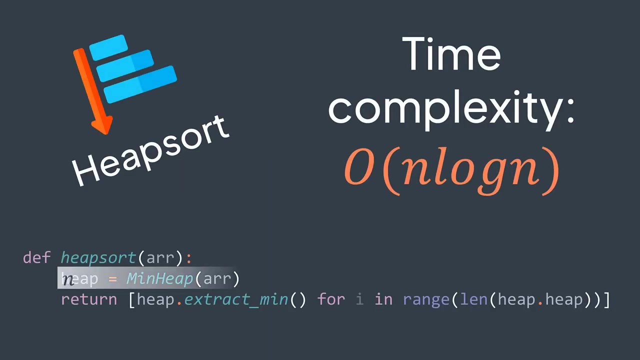 The time collector of hip sorts is hope and look at, because even if heapy fine CASOF Anna's shown earlier but calling extractman n times costs of and look and the time laxer of hip sorts is off analog. and because even if AP fine costs of anas. 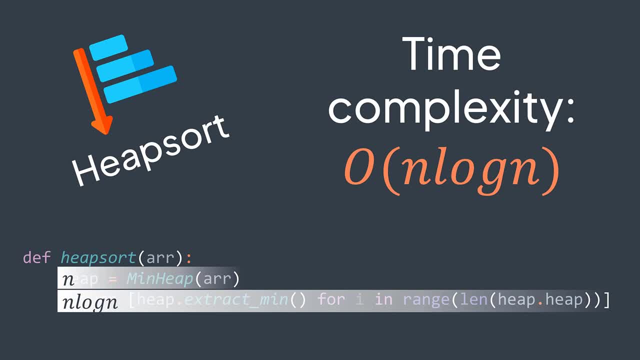 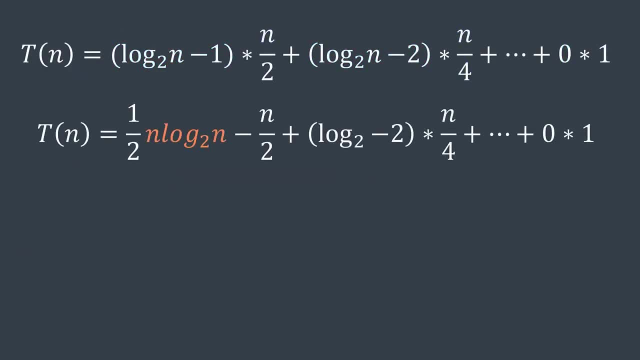 because extract main always call sift down on the root and the root is far from the bottom. So the first and by two extractions may require locked off and minus one iterations will really have the analog and turn. it will lead to an off analog and time complexity for heap sort. 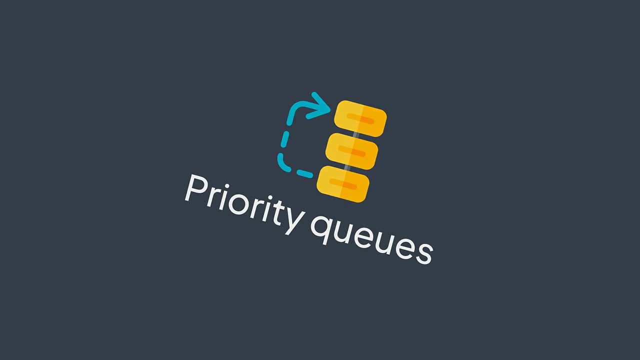 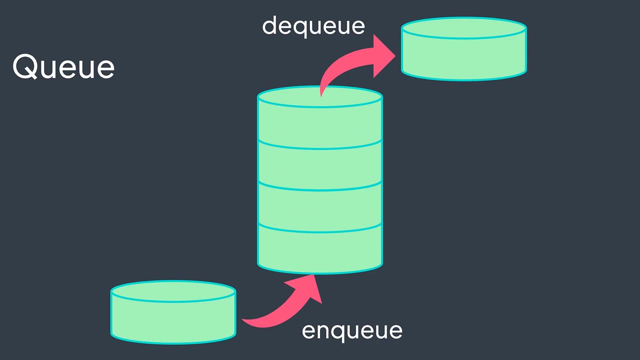 The second application is a priority queue. you probably know the queue data structure, data structure that works on the first in first out principle, where an element enters from the back and goes out from the front, But in a priority queue elements have a priority related to them. 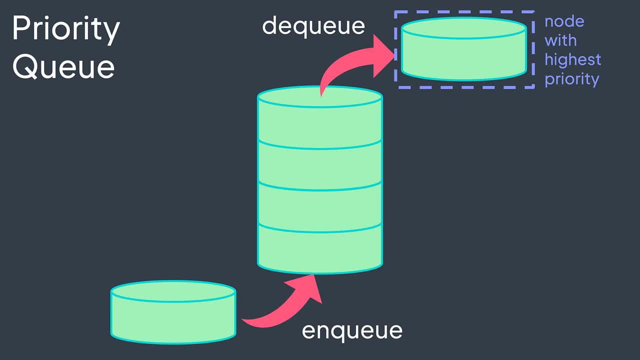 And we want the element with the highest priority comes always in front. who can implement the structure? with a linked list or an array? But one of the best implementations is by using a heap because of the low time complexity of its main operations. So in reality our priority queue will just be a heap, either mean heap or max heap. 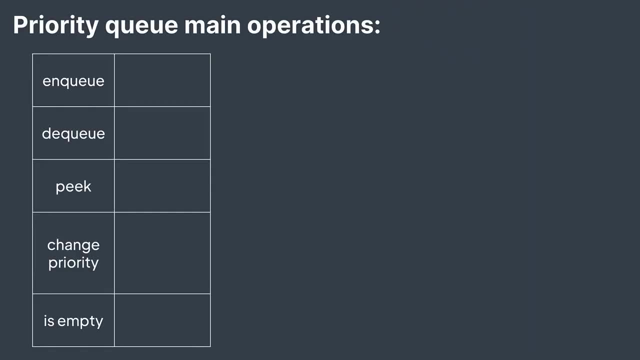 Main operations of a priority queue are in queue DQ, peak, which returns the element at front change priority and is empty, which says if the queue is empty And because we're using a heap and Q is done just by inserting the element in the heap. 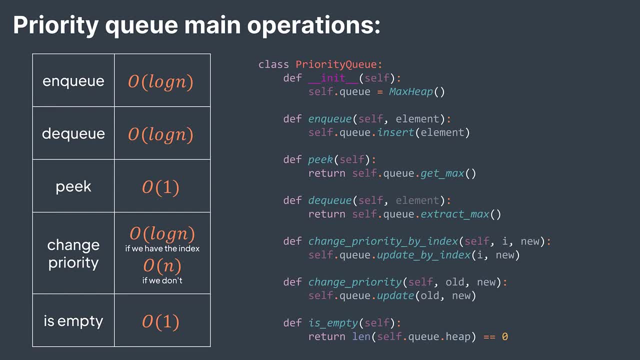 DQ is done by extracting max in case of a max heap peak. is done by returning get max in case of a max heap change. priority is done by using update and is empty is done by just checking if the length is equal to zero and we finished implementing the priority queue. 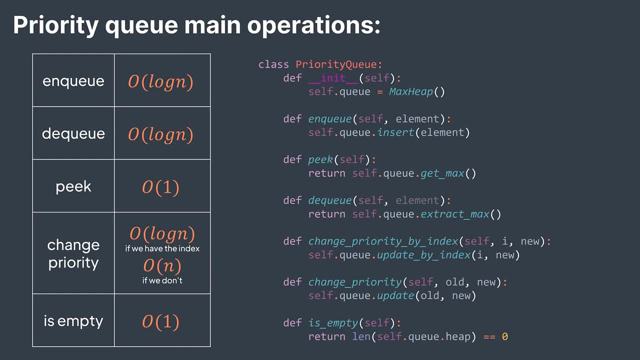 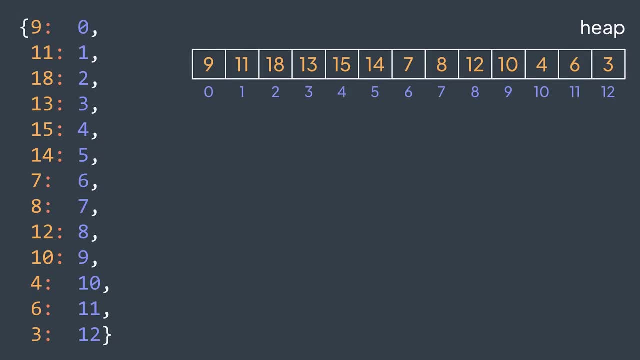 Note that to have the index and be able to change priority and off log- and we may need to use another structure to keep track of each element and its index in the heap. Also know that there may exist a library for priority Q- new language, to avoid reinventing. 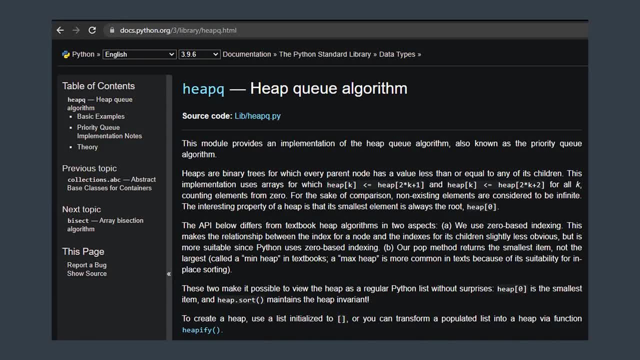 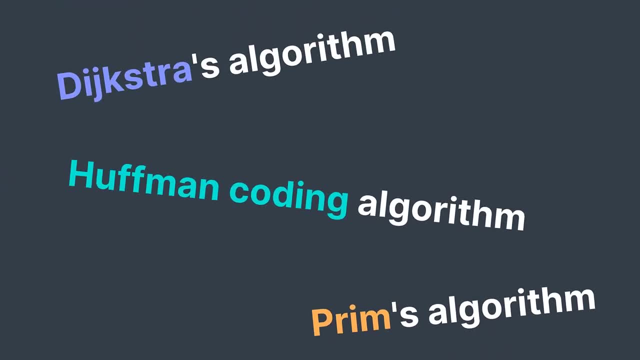 the wheel. For example, in Python there is heap queue And the priority queue has many applications. we can use it in the extras algorithm, half man coding algorithm, preempts algorithm and many other ones. we will see them in future. 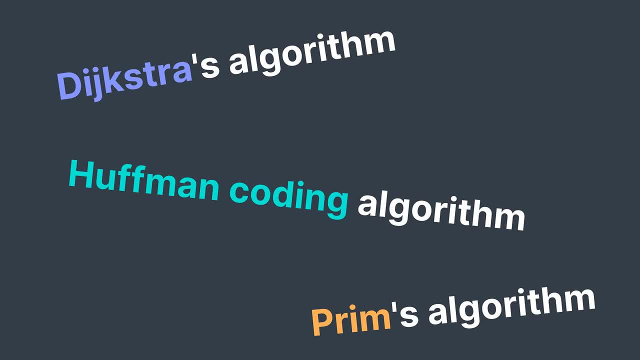 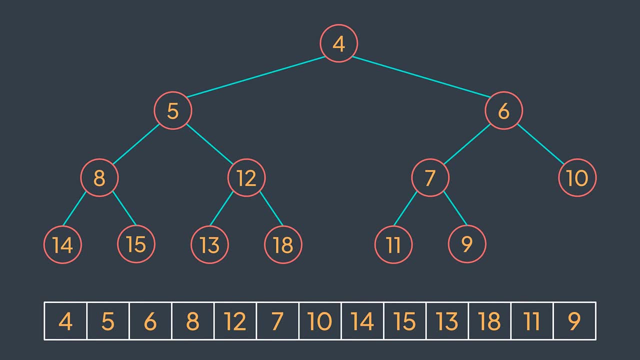 videos. We reached the end of this video. in this one, we discovered the heap data structure, its advantages, its implementation and some of its applications. I hope that you understood all of this. please subscribe and share this video and see you. in the next one.